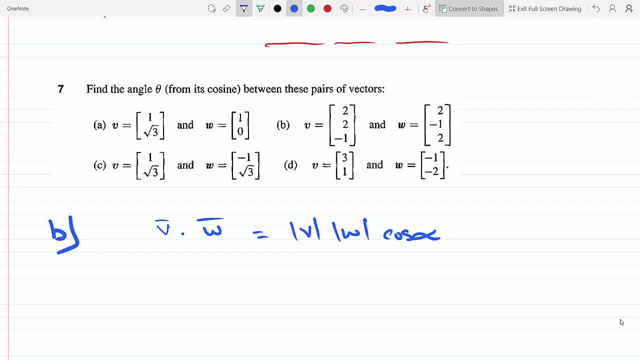 W times cosine, the angle alpha between them or theta. The question calls it theta, It's called theta. So this is V, this is W and this is the angle between them. So now we know that the magnitude of the vector. this is going to close on me, I apologize. 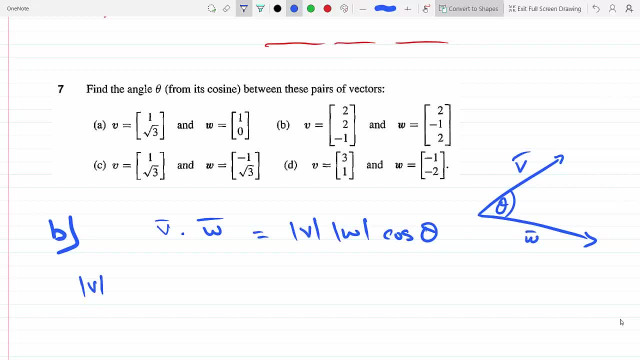 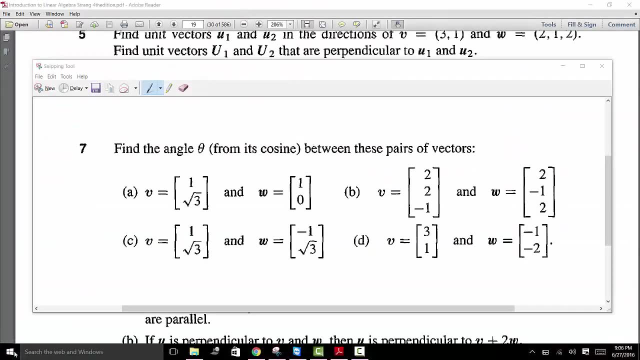 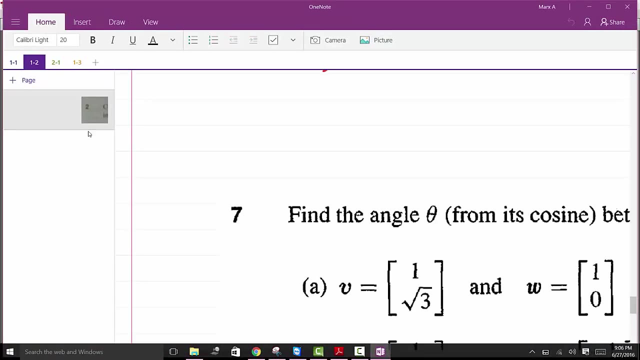 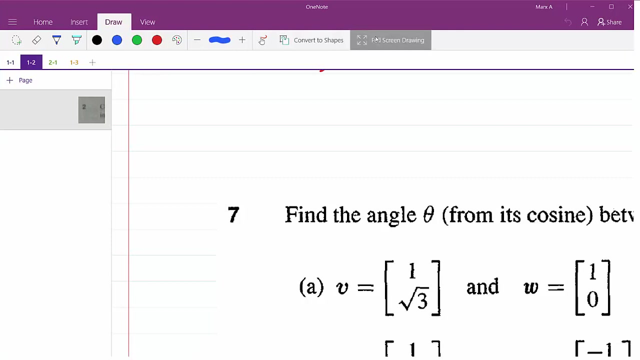 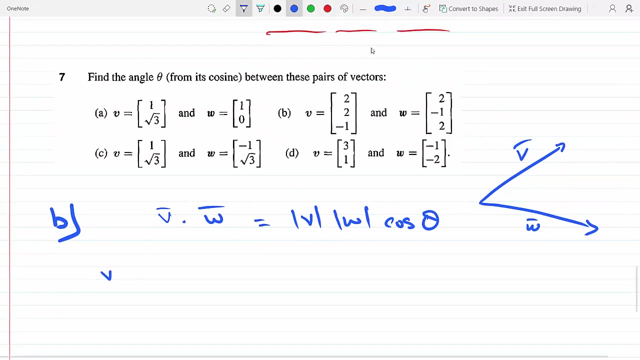 Wait for it to close and reopen. Okay, we know that the magnitude of the vector is technically the: how long the vector is. It's the sum of this, the square root of the sum of the squares of its components. Another way to say it is: it's dotting the vector with itself. So the magnitude of V. 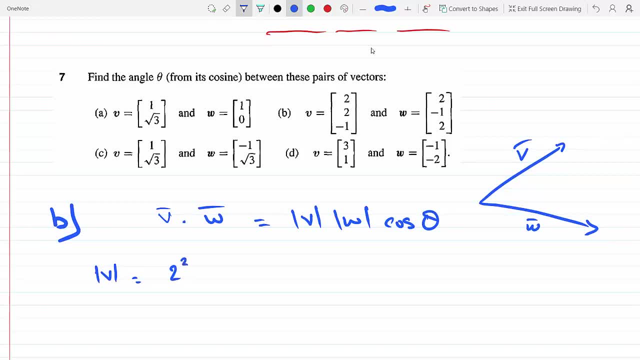 will just be. so I'm doing part B: 2 squared plus 2 squared plus 2 squared, Or sorry, the third one is minus 1 squared, And so that would get us 9 square root 9 is 3.. Same thing for W. 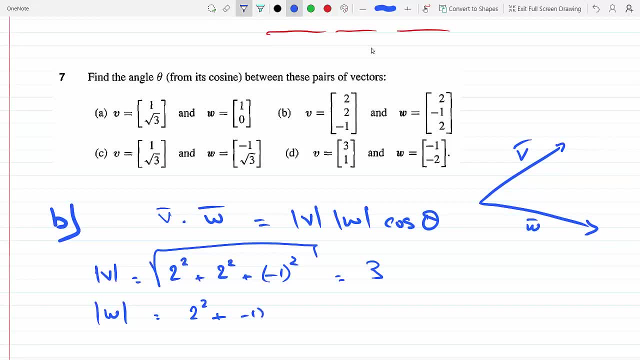 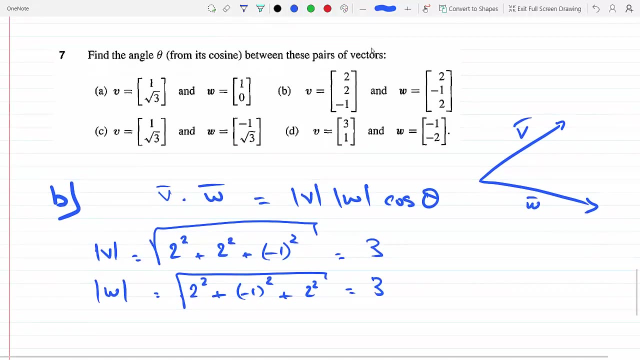 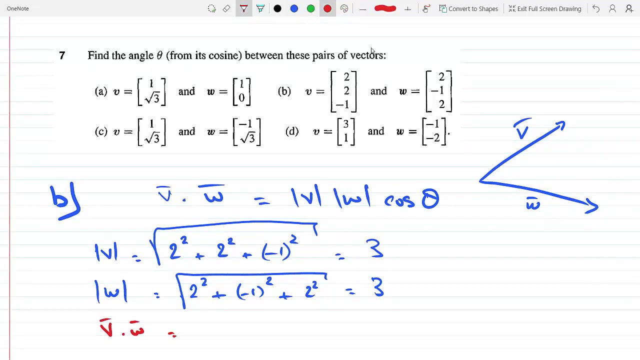 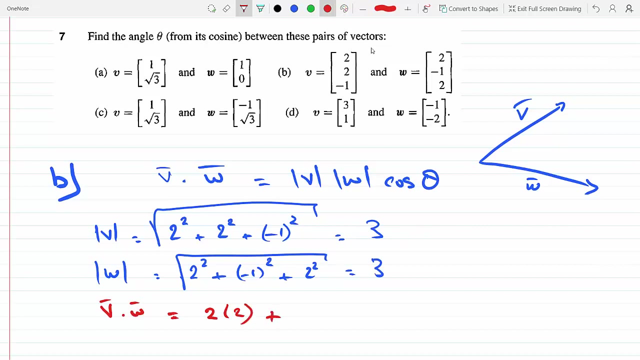 We get 2 squared plus minus 1 squared Plus 2 squared. Different order, but they're the same numbers. So 3 as well. And now we do the dot product between these two vectors. So V dot W. So it's the multiple, it's a scalar quantity and it's the multiplication of the corresponding components. So it's 2 times 2 plus 2 times minus 1 plus minus 1.. 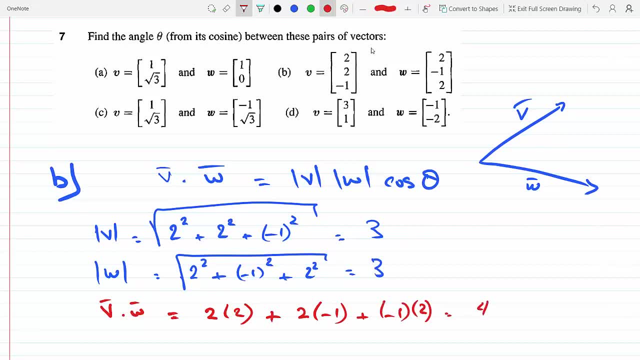 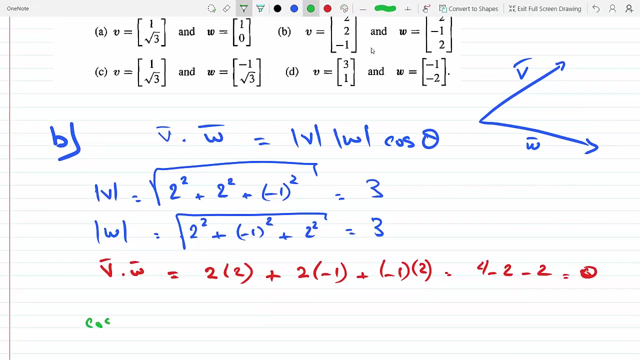 1 times 2.. So what's that? 4 minus 2 minus 2.. So that is 0.. So we know that if, if the two dot products is 0, we know what the answer to that is. That just means that the two vectors are perpendicular to each other. Since the answer is 0, as can be illustrated by cosine, theta will just be the dot product over the magnitudes. 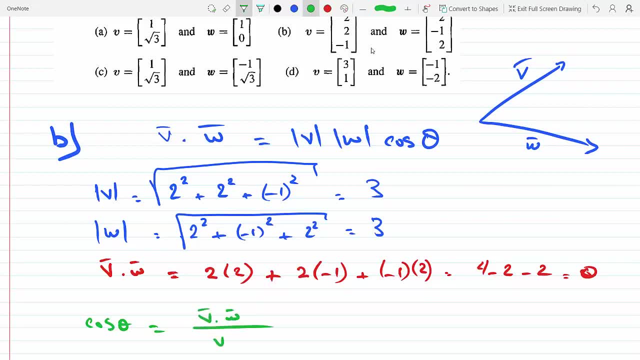 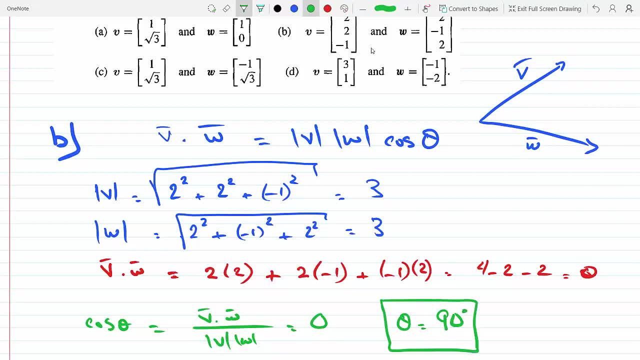 these two vectors are orthogonal. that does it.